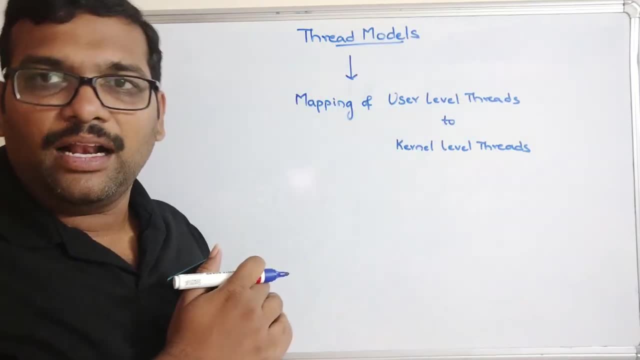 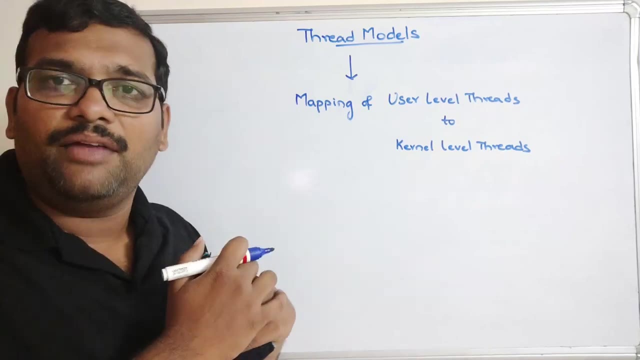 are going to map the user level threads to kernel level threads. So here the second question question is: so what is the reason why we are mapping the user level threads to the kernel level threads? because so, as we discussed in our previous session, the user level threads 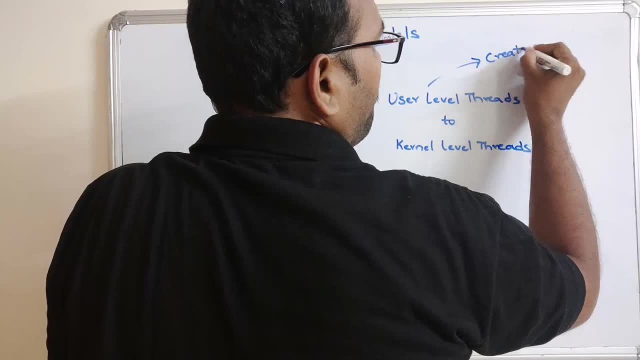 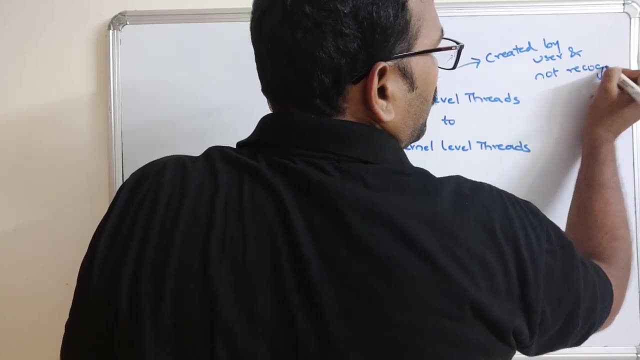 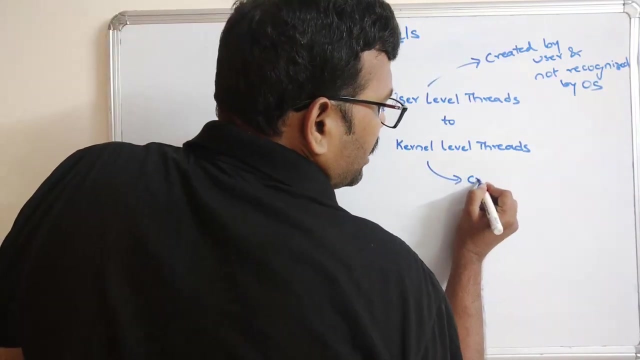 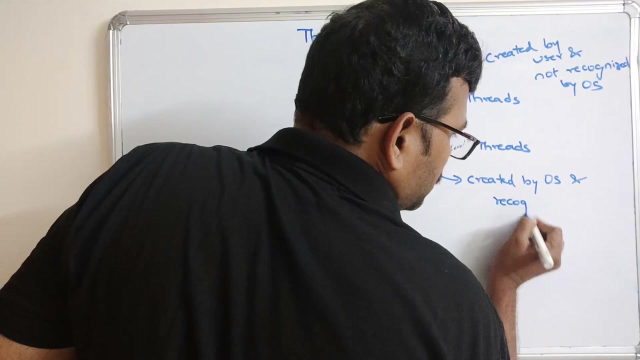 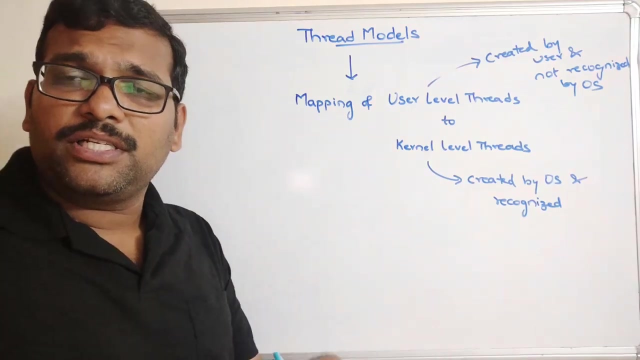 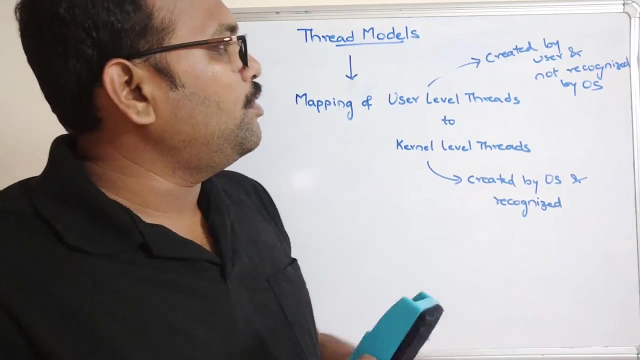 were created by user and not recognized, not recognized by operating system, right. whereas the kernel level threads created by operating system and recognized, okay, and recognized because they are created, right, recognized. so whatever it may be, either process or a thread, it should be get executed by the process itself, right? so, without recognizing these, 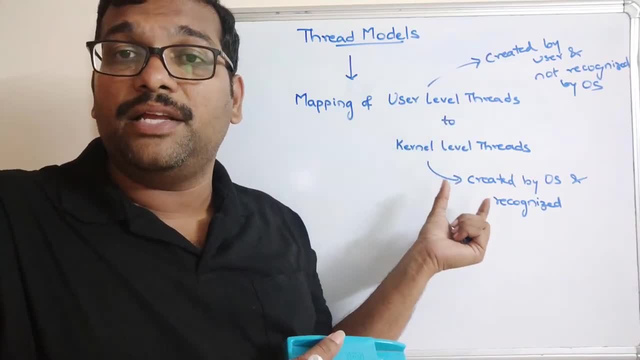 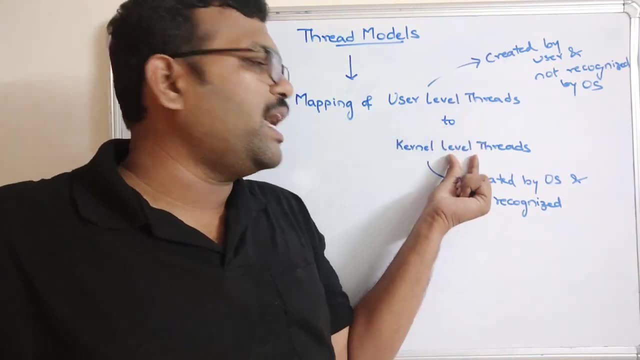 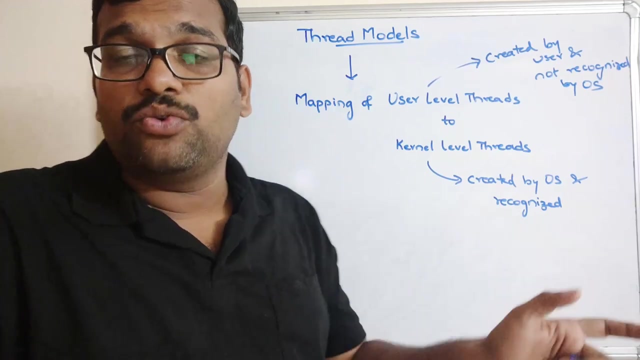 user level threads how these threads will being executed by the CPU. So that's why we are going to map these user level threads to the kernel level threads in order to get executed by the CPU. so here the CPU is a processor, right, so everything should be executed by the processor, so only the processor can recognize the kernel level. 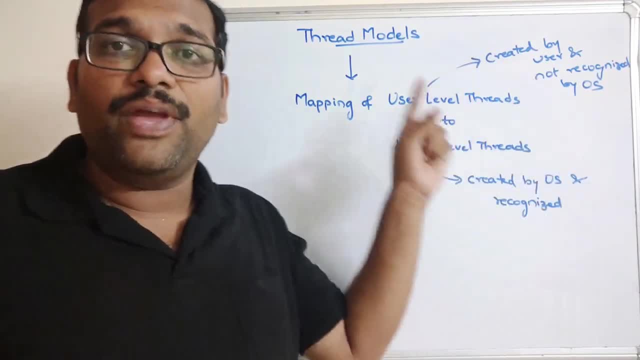 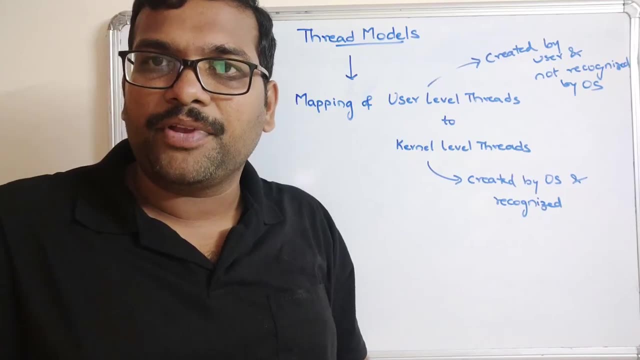 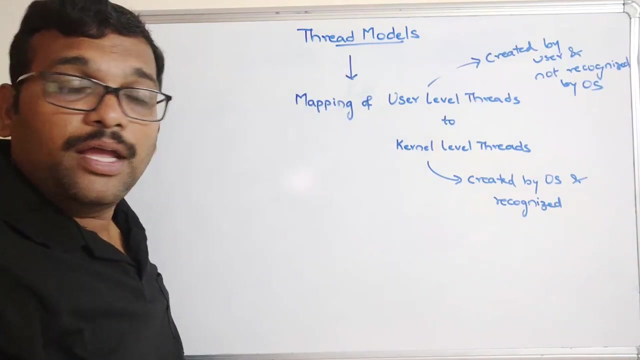 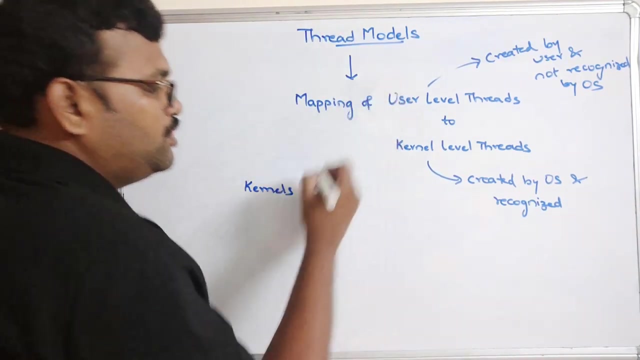 threads. they can't recognize the user level threads. so that's why we have to map the user level threads to the kernel level threads in order to execute these user level threads. right, and this process, This mapping process, is called thread models. okay, and these kernels, the kernels which are 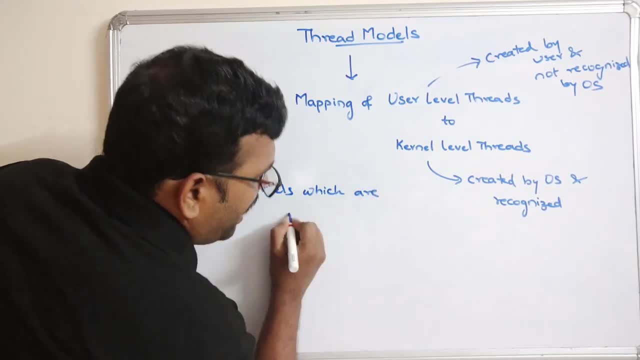 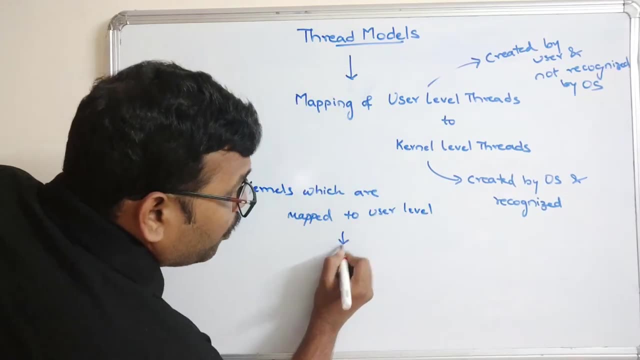 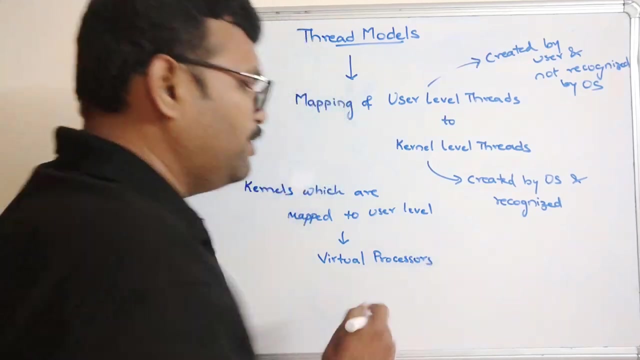 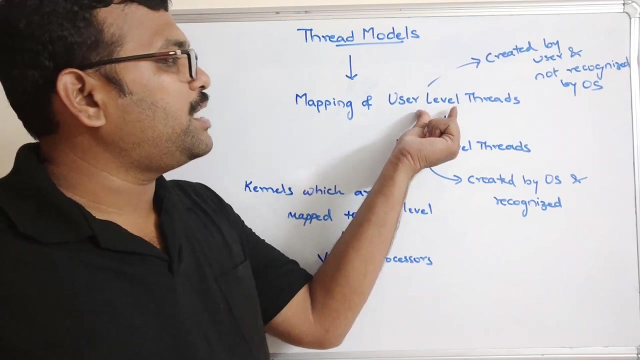 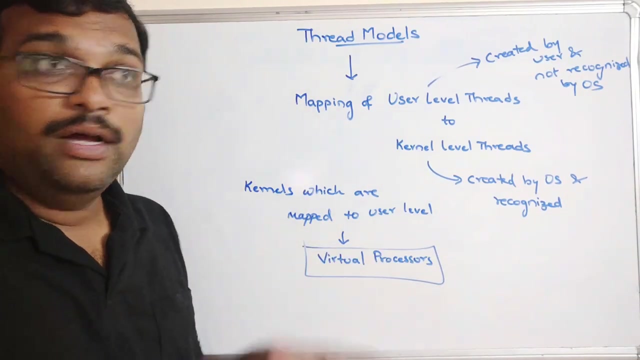 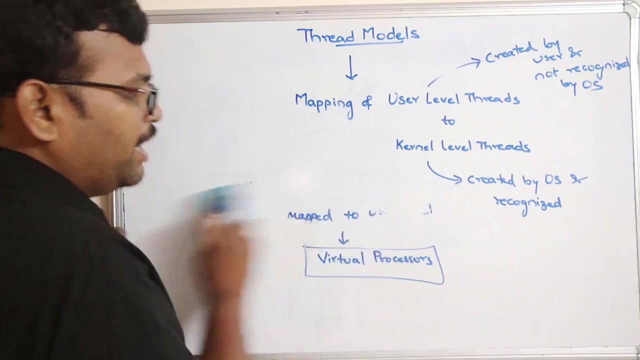 mapped, which are mapped to user level, are known as virtual processors- virtual processors right. These kernels are being created by the operating system and we are mapping the user level threads to these kernels. so these kernels we call it as a virtual processors right. so these user level threads are being executed by the virtual processors. now there are three different. 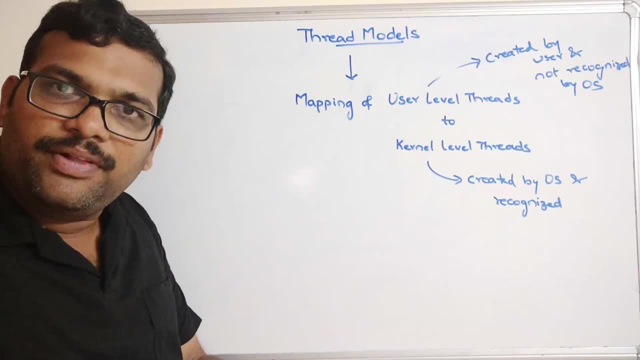 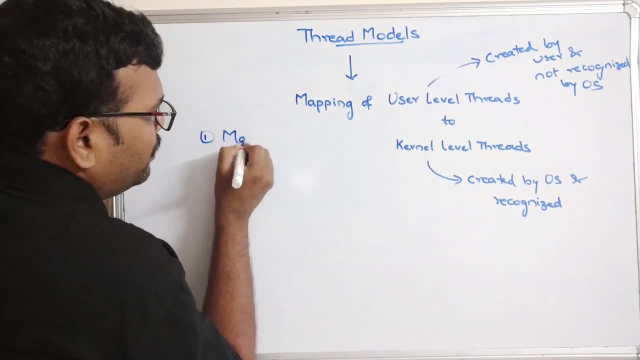 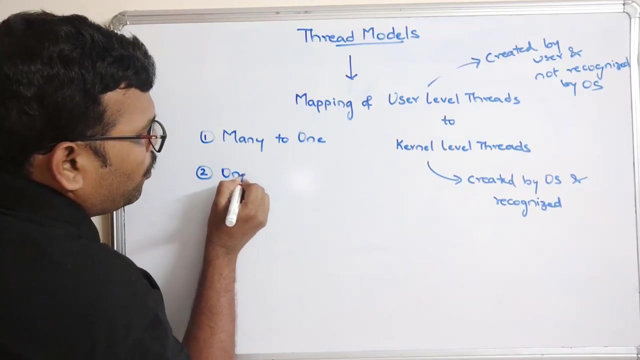 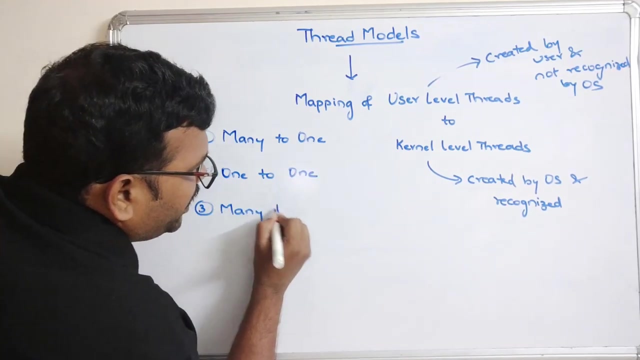 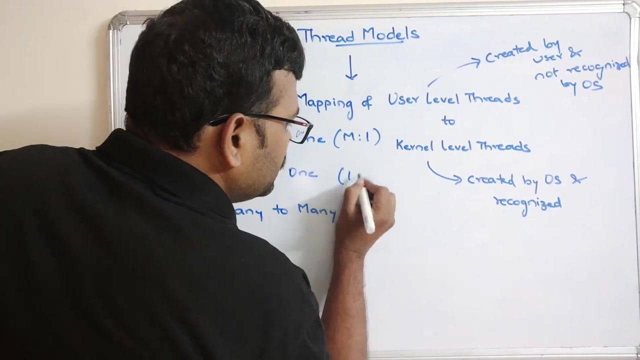 thread models to map user level threads to kernel level threads or to execute the user level threads by the processor. The first model: many to one, many to one, and one to one and many to many. so simply we can call it as m to one and this is one to one and this is m to m, m to m. so this is m to m. 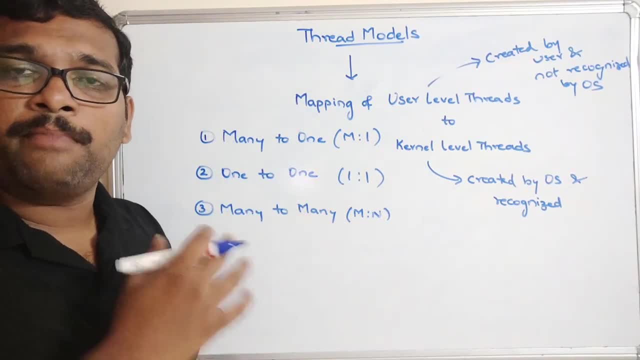 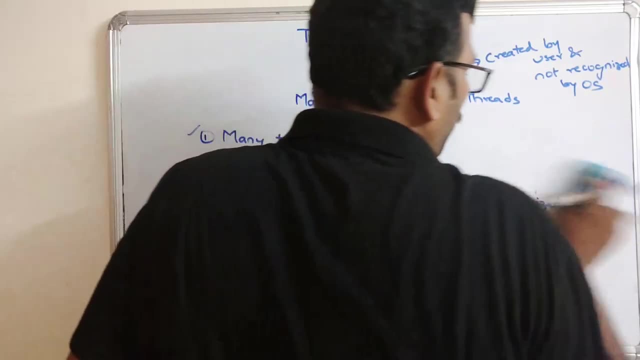 So these are the three different models which are used to map the user level threads to kernel level threads. So we will see one by one Coming to the many to one, So in this many to one. so there are different threads, right. 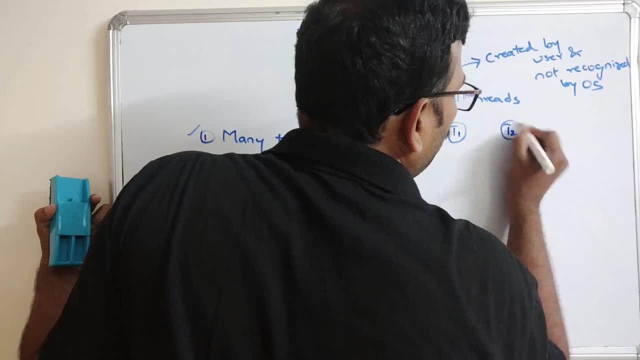 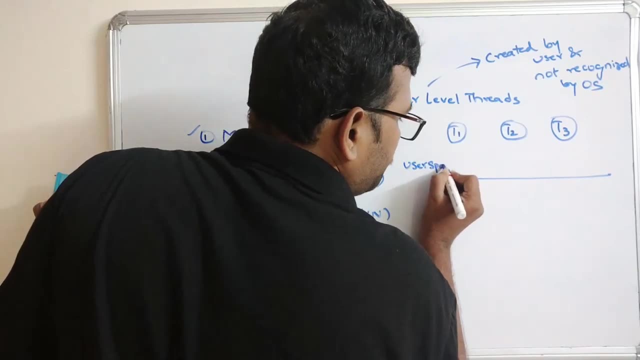 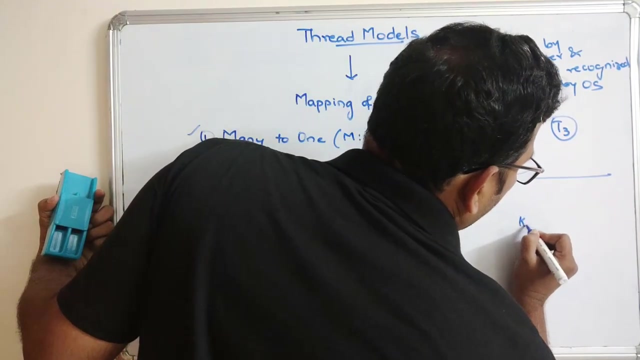 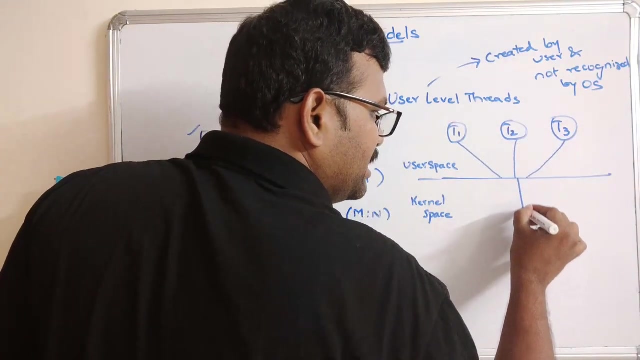 So thread one, thread two, thread three: right, So this is a user space, user space and this one will be the kernel space. kernel space, That will be some K1.. So these threads are being mapped to a single kernel. 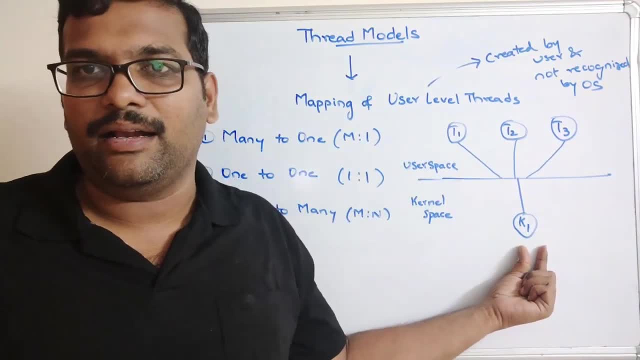 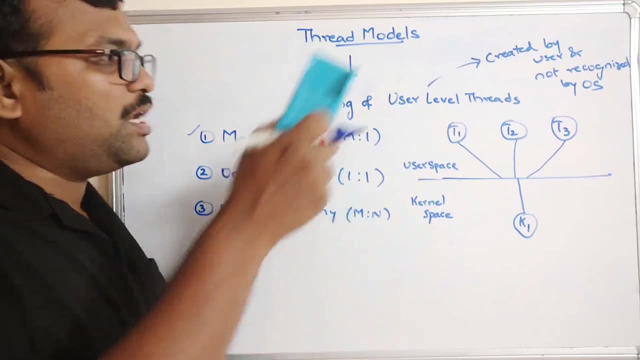 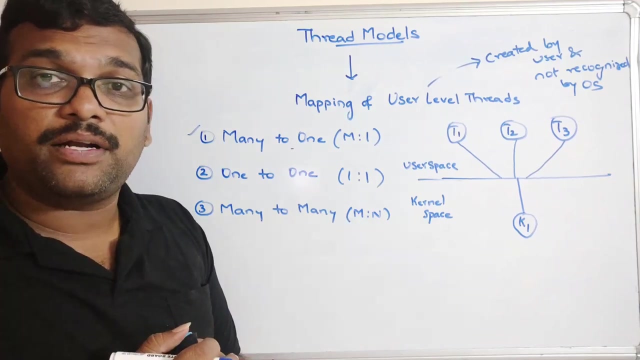 All these threads will be mapped to the single kernel. So this type of model we call it, as in many, to one, That means many user level Threads will be mapped to the single kernel. So everything is fine. But there is a disadvantage of using this model. 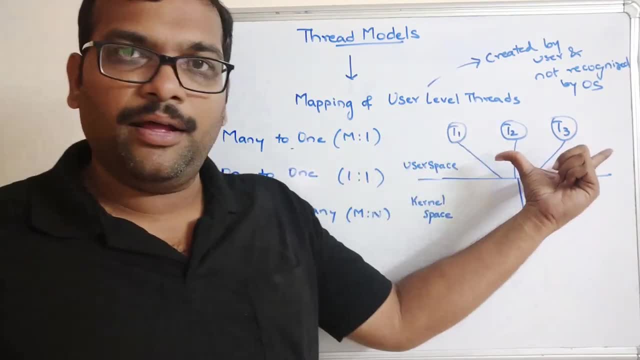 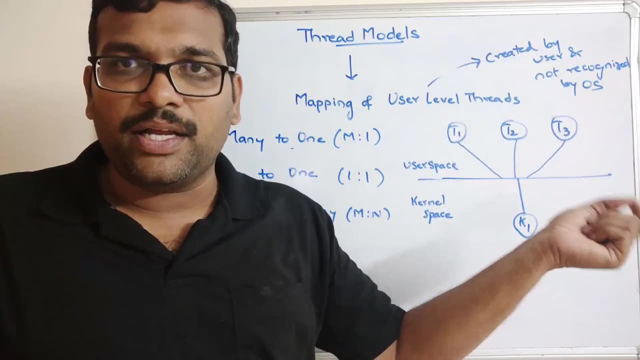 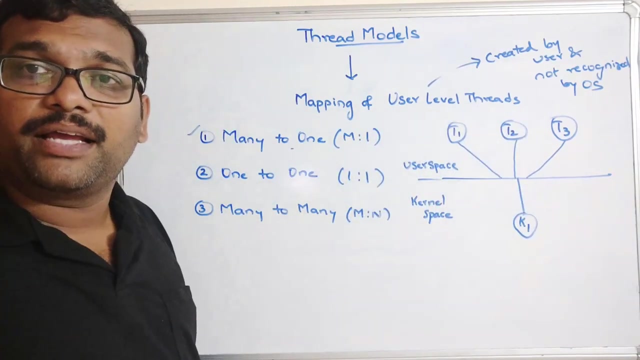 What is the disadvantage If any one of the thread, if any one of the thread is being waiting for any IGO operation and if it is moving towards the blocking state immediately, the complete process will be in the blocking state, So no other thread will be executed by the kernel. 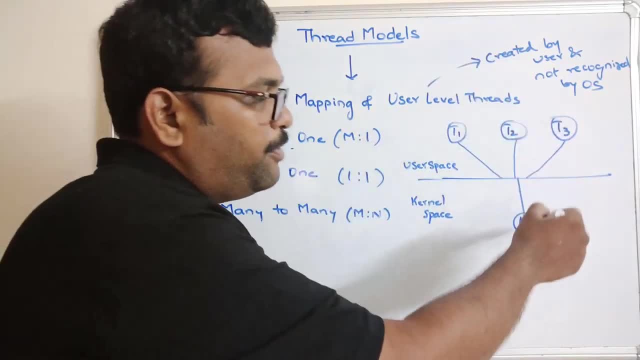 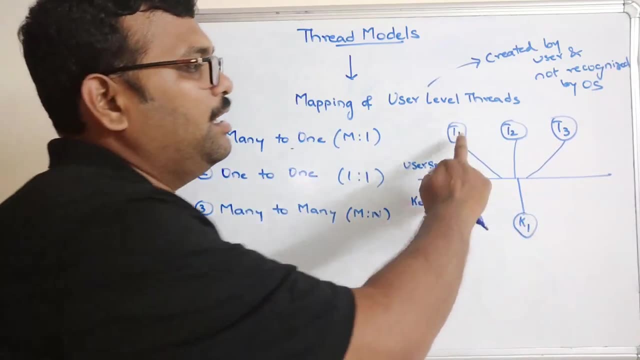 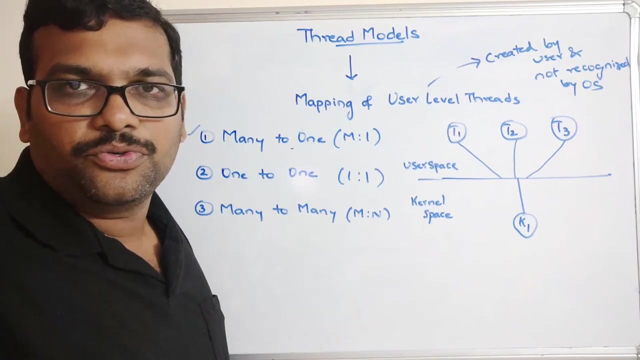 Because all the three Threads are being mapped to the kernel. So if any one is in a blocking state, so the remaining threads have to wait until the block- I mean the thread which is being blocked- should be being executed until it completes its execution right. 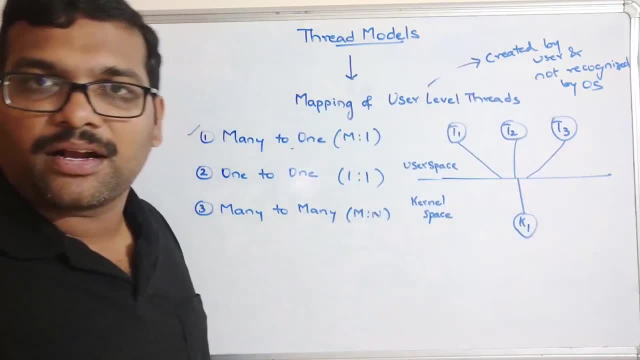 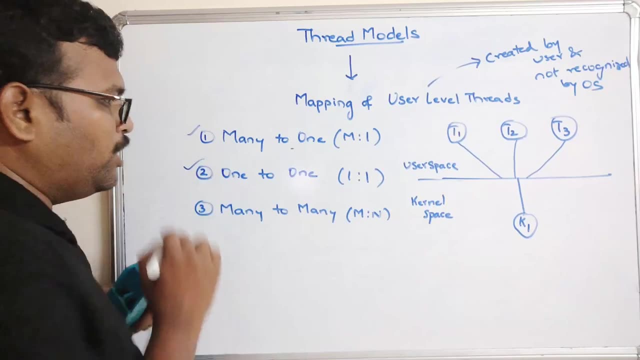 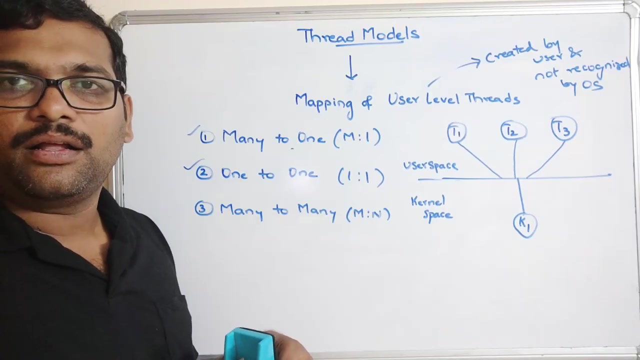 That's the main drawback, because all the threads mapping towards the same kernel itself. So in order to overcome this one- okay, in order to overcome this one- we are moving on with one to one. So in this model, One thread will be associated with the one kernel, right? 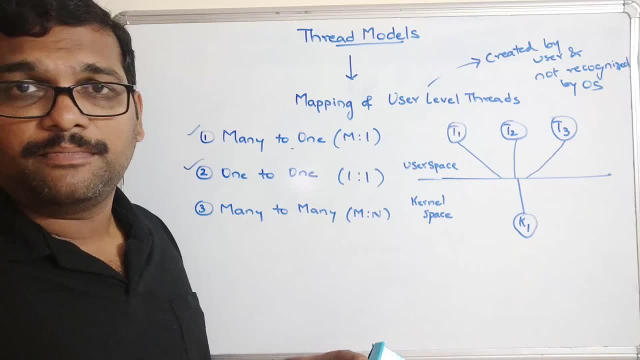 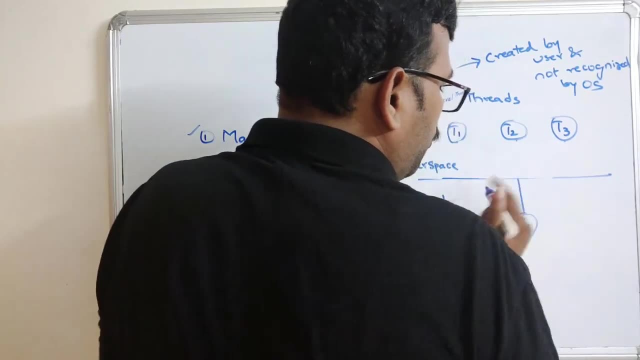 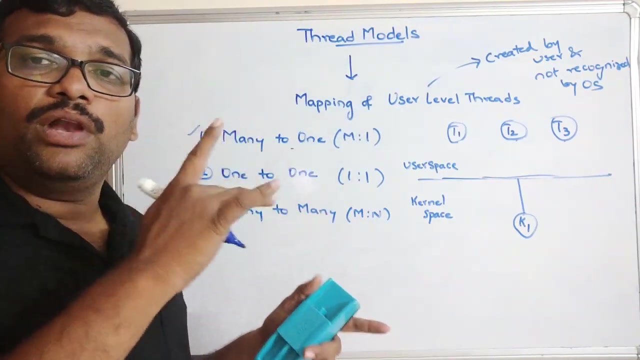 So here we are having a multiple virtual processors, So so hope you understood the disadvantage of using the first model, that is, many to one, So if any one. so mapping all the threads to the single kernel, So only if any one of the thread is in blocking state. 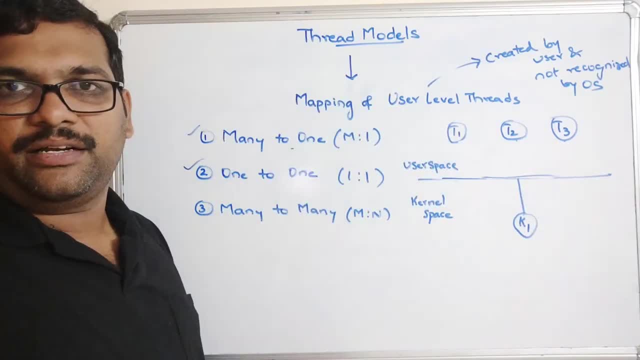 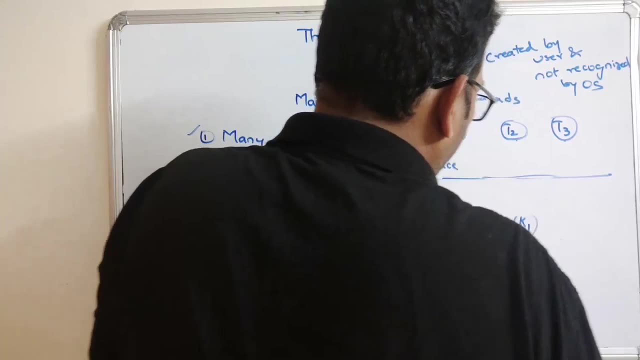 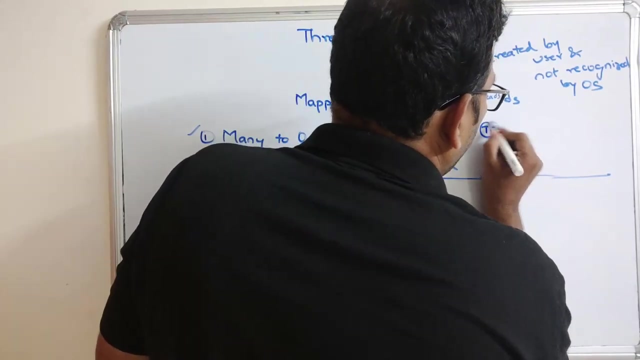 So all the remaining threads have to be in waiting state until it completes its execution, Because all have mapped to the same kernel And now see the next one. one to one, That means in order to overcome that one. so we are mapping each and every thread. 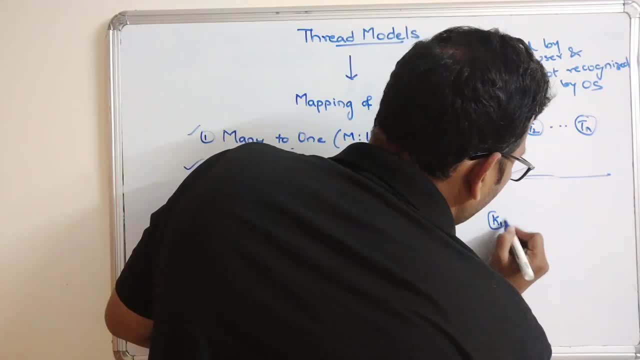 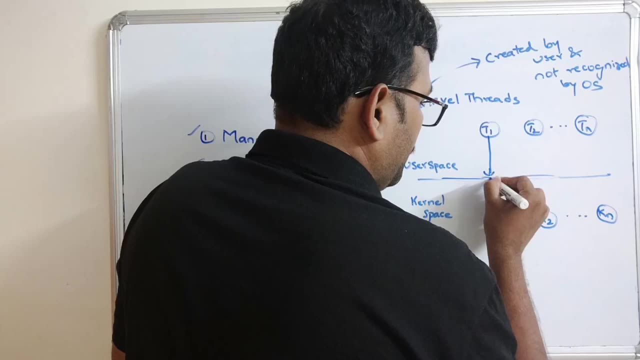 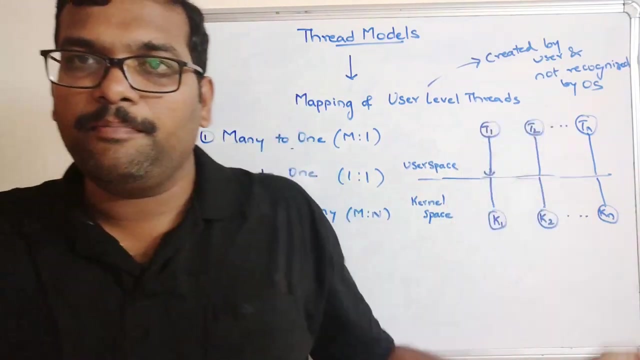 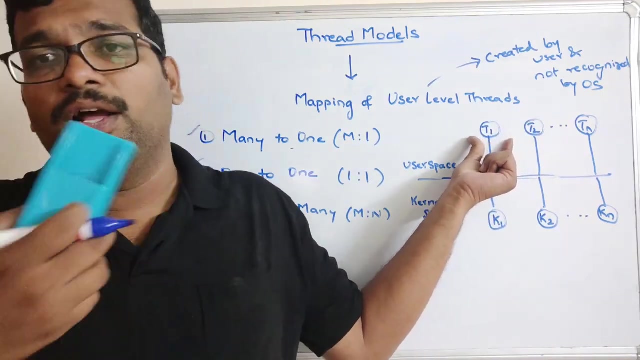 Each and every thread are mapped to each and every kernel. Each and every kernel, So every thread will be mapped to each and every kernel. So the problem has been solved. If T1,, if T1 is in a blocking state for waiting for any IOO operation immediately, T2 can't wait. 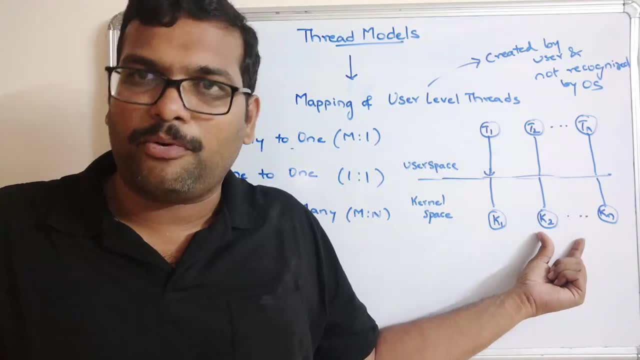 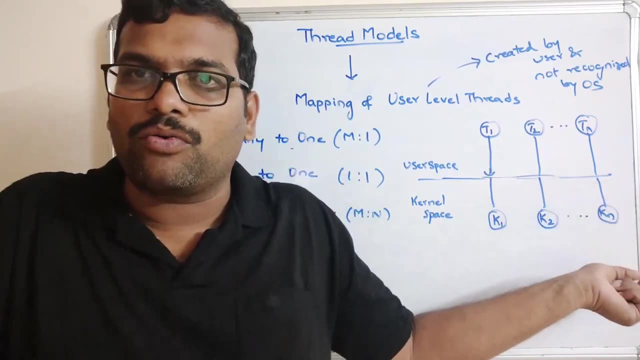 It need not to wait right, So T2 will be executed by the another virtual processor. So K2, right kernel And similarly T3 will be executed with one more kernel, right. So it overcomes the disadvantage. 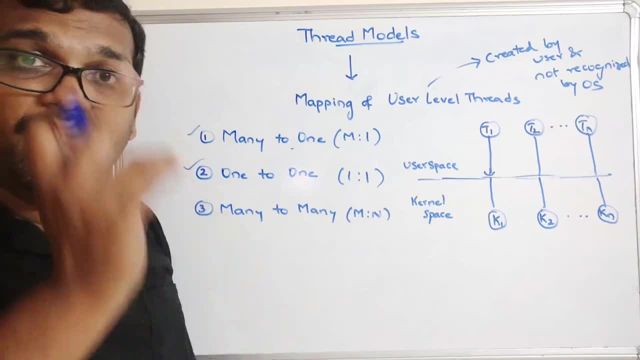 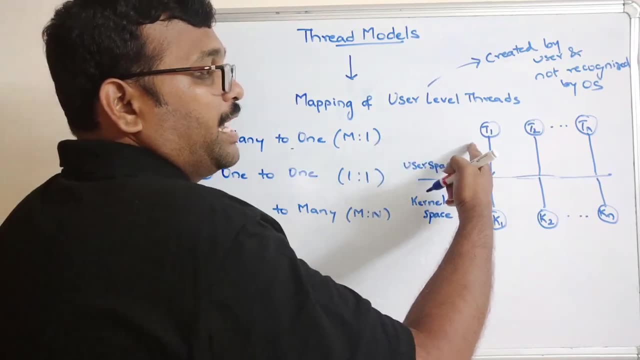 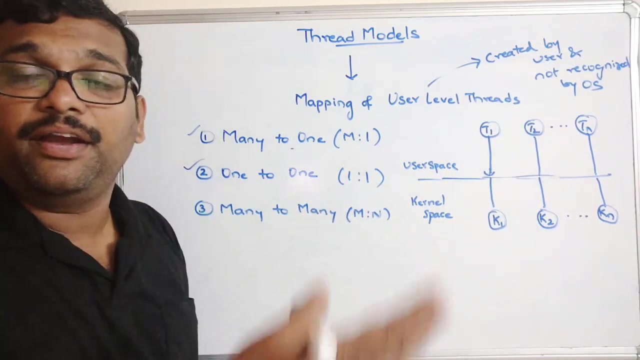 So it overcomes the disadvantage of first model, that is, many to one. But here in this model again, we are having some disadvantage. What is the disadvantage? So the number of threads are being increased automatically. The number of kernels are also being created, right. 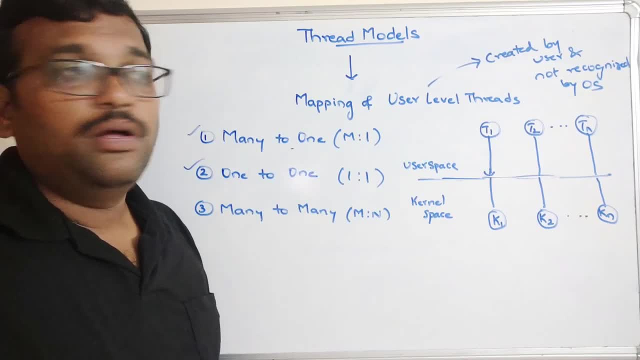 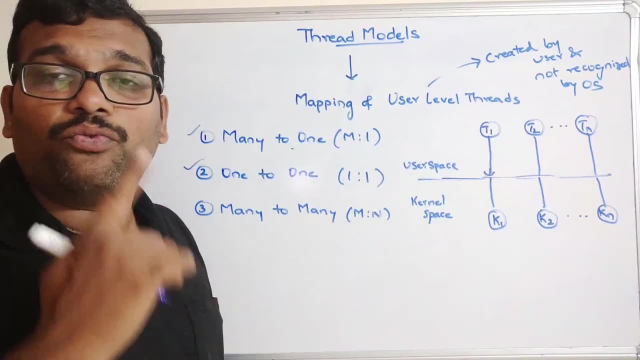 So we have to create a more number of kernels. So if a process is having some 10 threads, so there should be 10 kernels, Because one thread will be associated, So we can create a more number of kernels. So that is the main drawback. 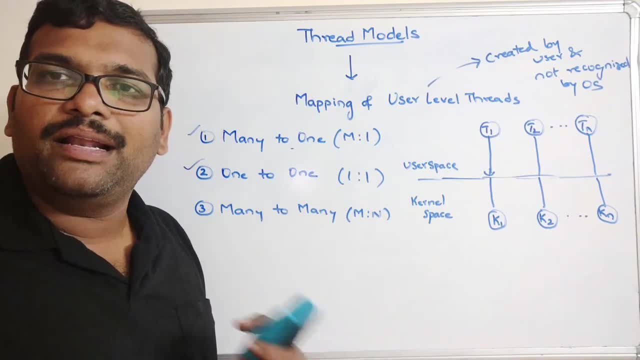 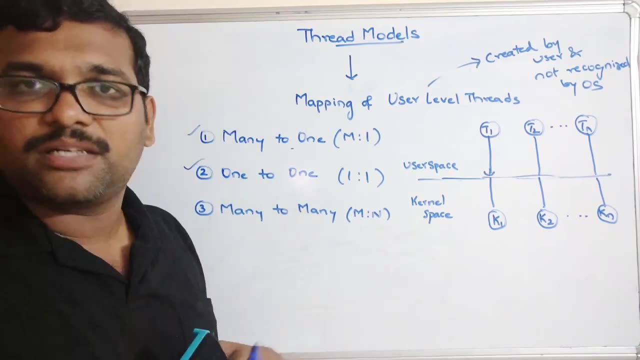 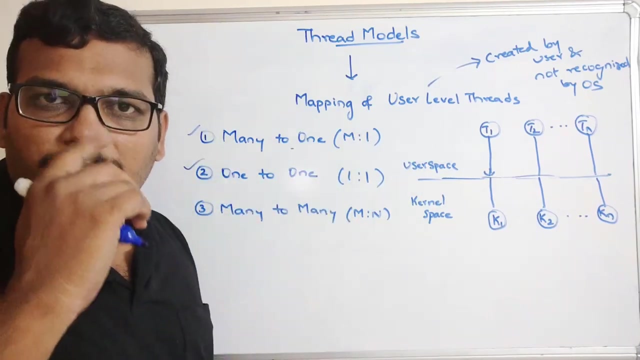 Because so creating more number of kernels automatically reduces the performance of processor. So the kernel will be created by the CPU by using some system files, right? So creating more kernels automatically reduces the performance of the processor. So that is the main drawback. 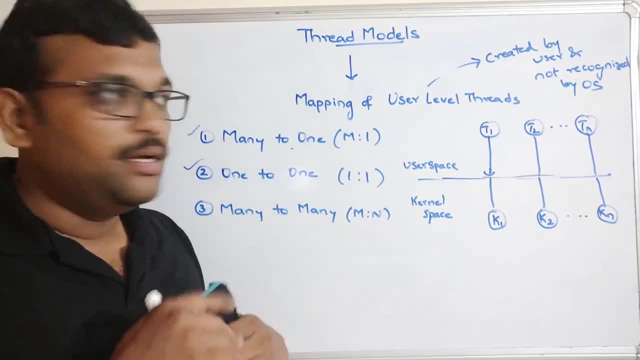 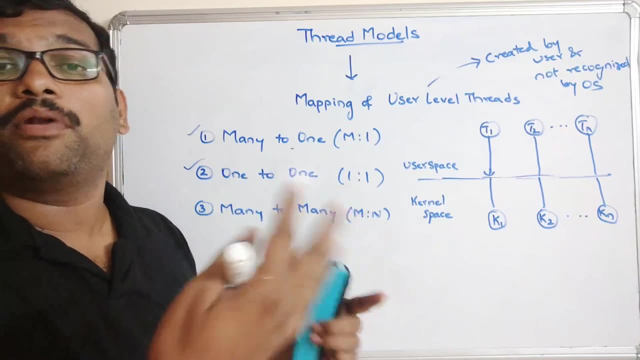 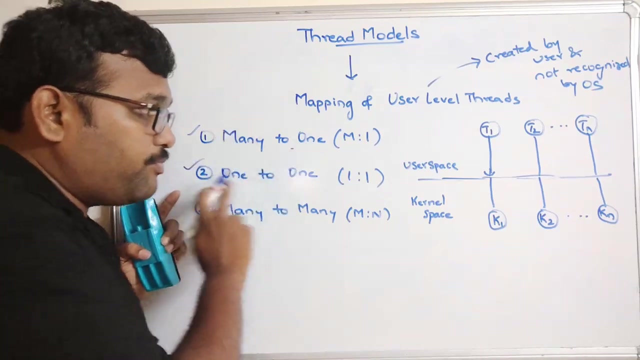 So it overcomes the drawback of first model. That means the waiting state, right. But here there is a one more drawback fact, that is, more number of we have to create a more number of virtual processors. so in order to overcome the second disadvantage- i mean that's a disadvantage of second model- we are moving with- 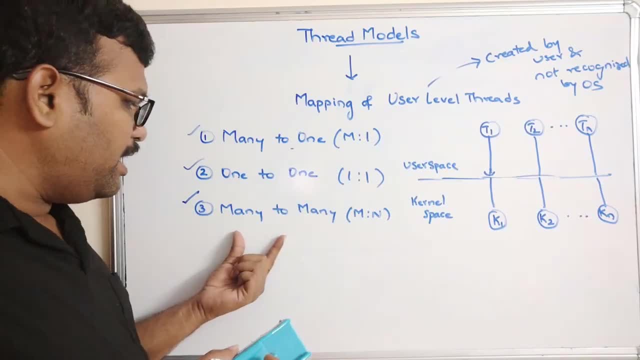 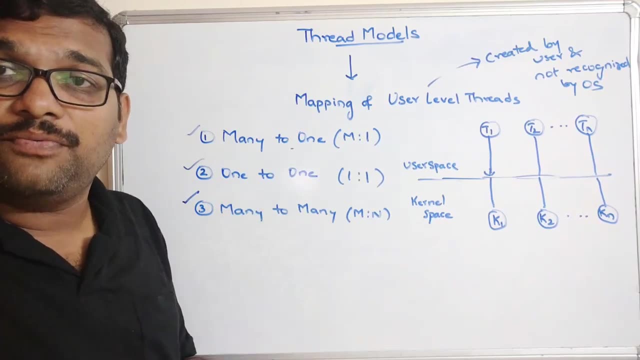 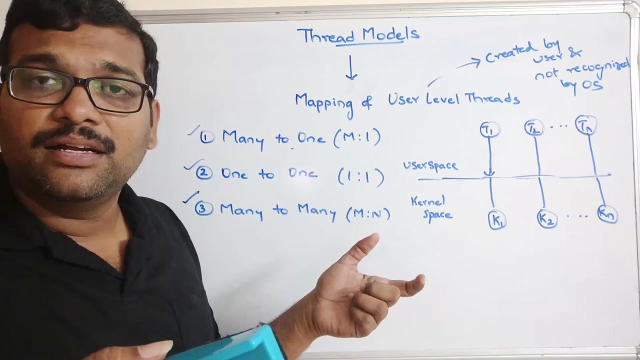 the third one, which is an efficient one here: the relay, the mapping, is between many to many, so m number of threads will be associated with m number of kernels, so there will be a pool of kernels. for example, there are 10 threads, so we can create a 5 kernels and 10 threads will be. 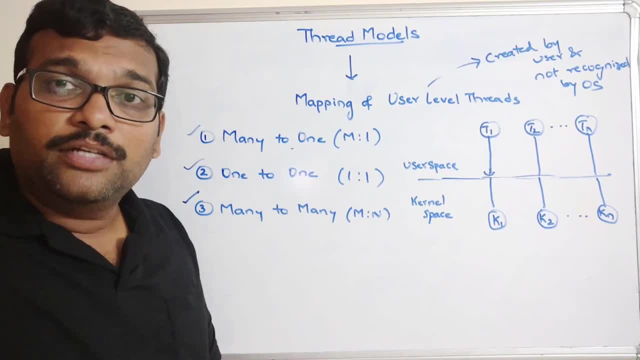 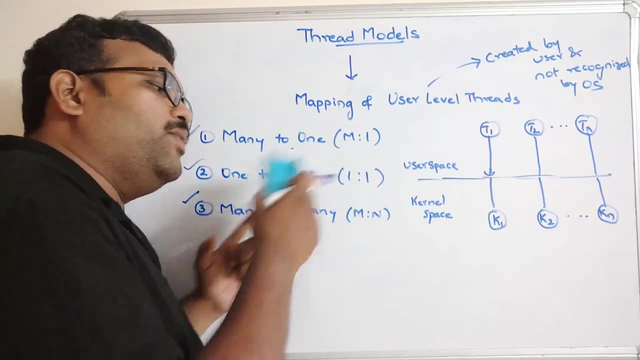 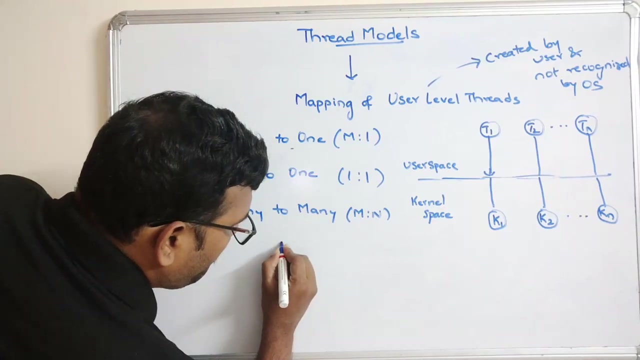 mapped to the 5 kernels, right? so we need not create a 10 kernels each for one thread, right? so here, if 10 kernels, if 10 threads are there, we can create some less than n kernels, right? so if there are m threads, then automatically we can create. 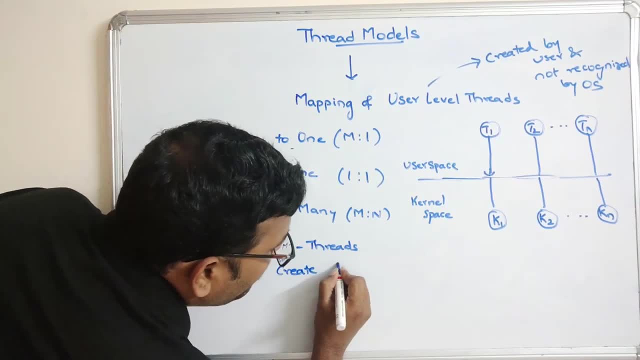 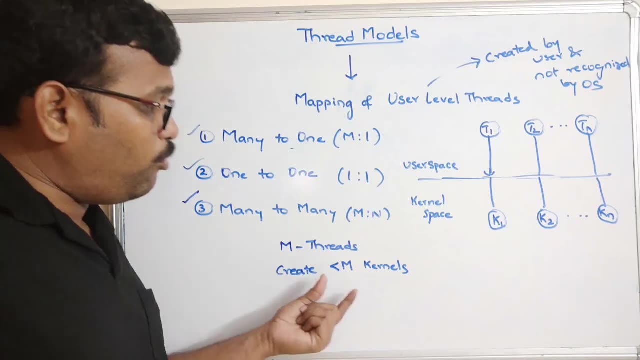 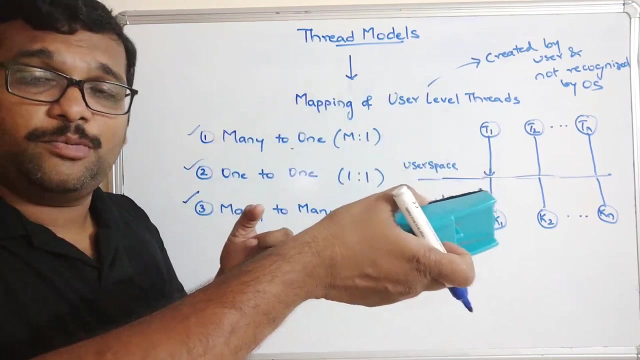 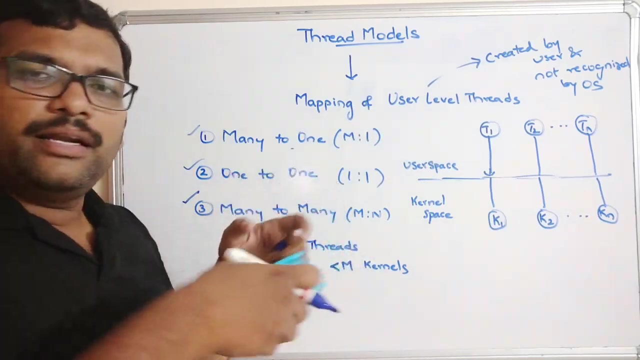 m. we can create less than m kernels, less than m kernels, so automatically. that avoids the disadvantage of first one. that means if any one of the process is in a waiting state, automatically the next process can continue its execution with associating with the another kernel and the second one. so it is not necessary to create a more number of kernels. 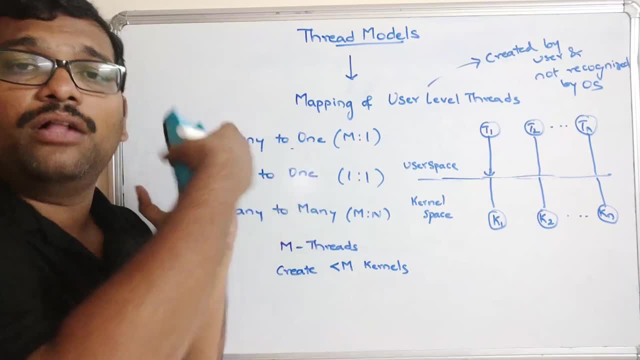 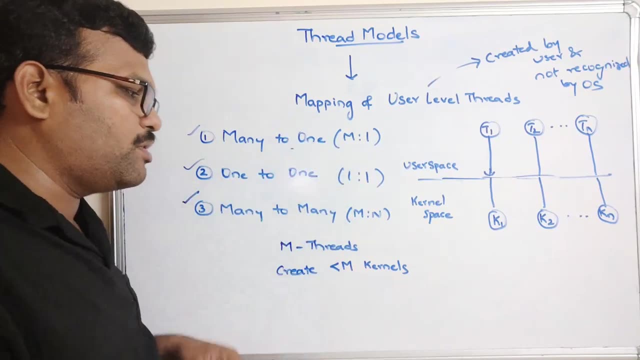 some sort of kernels can be used and we can assign all the kernels to the next kernel so we can create a more number of kernels. so again, we are adding all the threads to those kernels itself, right? so these two disadvantages of both the models can be overcome in this third model. so this will be then efficient one. 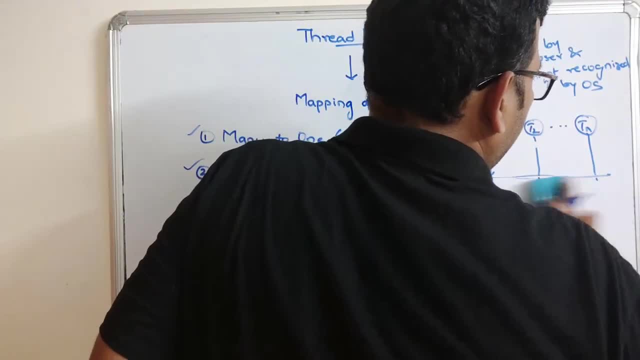 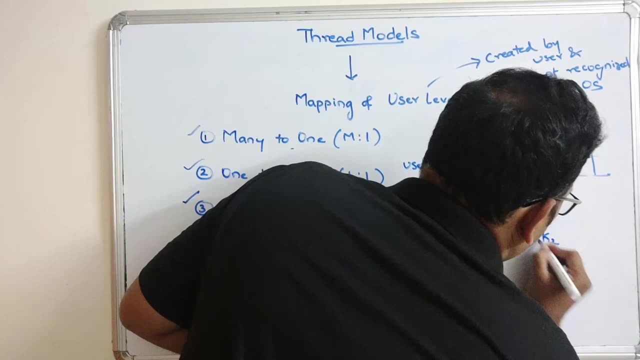 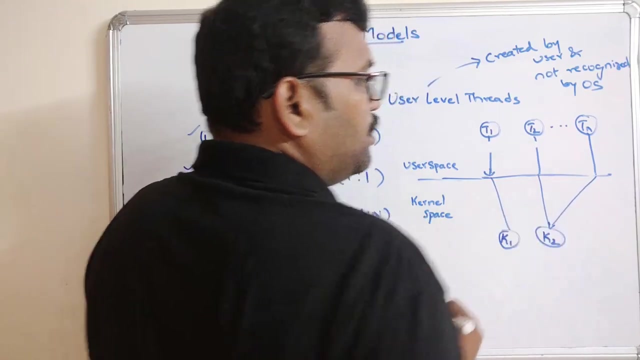 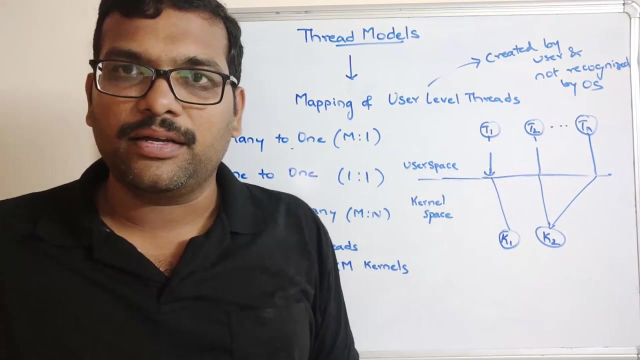 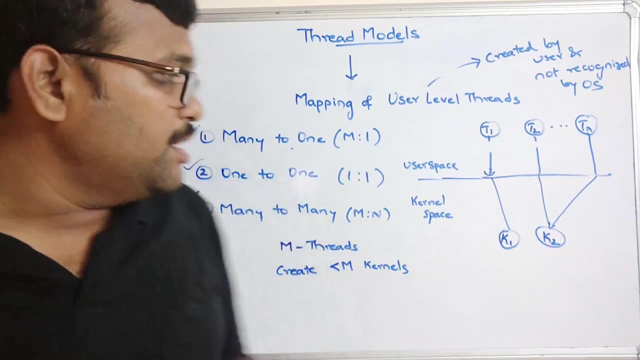 so here, let it be so: k1, k2- Ok, so, so like this, we can assign the memory of models okay, kernels, okay. we can map the threads to the kernels. so it is not necessary to map every thread to every kernel, right? so this is how the kernel- i mean user level threads- are being executed.